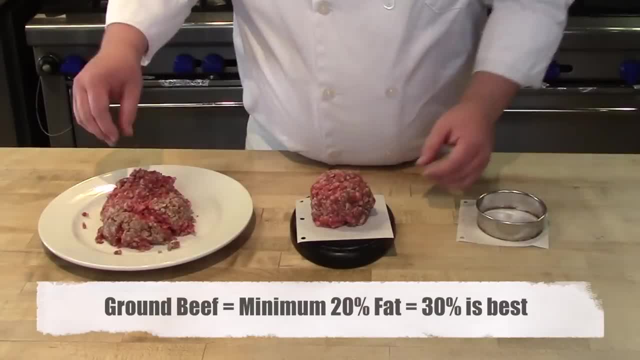 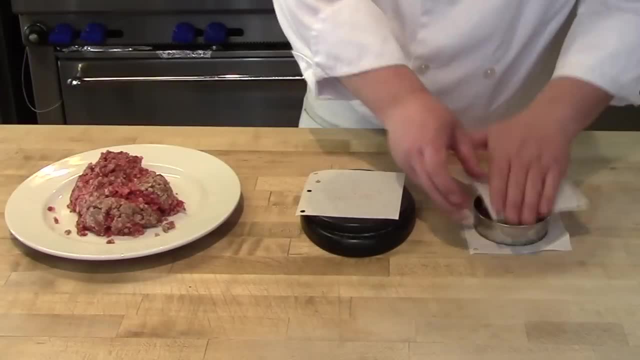 70% lean, 30% fat. That fat ratio is going to keep it moist and flavorful during the cooking process And I'm weighing out an eight ounce ball. I'm going to place an eight ounce ball into a four and a half inch ring, mold and gently press down using parchment paper. That's it, It's done, It's. 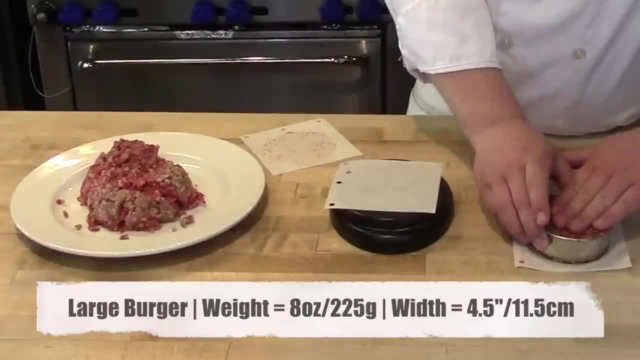 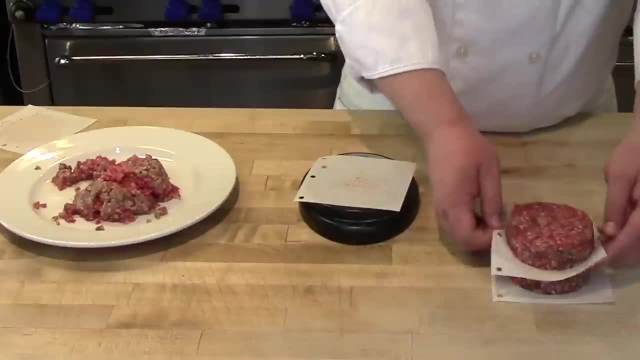 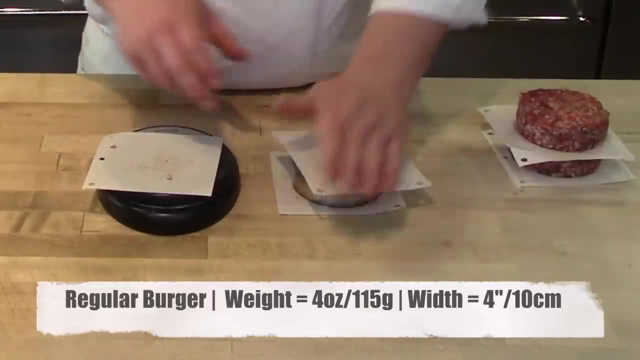 formed. That's our eight ounce steakhouse burger patty. Okay, now, if you want a more reasonable size burger, your standard burger size is going to be four ounces And we're going to do four ounces weighed out of our ground beef into a four inch ring mold and then press down using parchment. 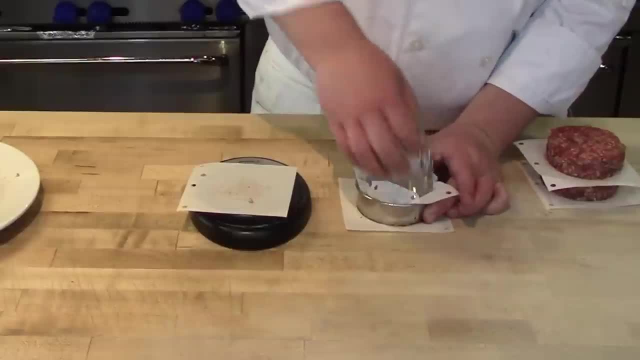 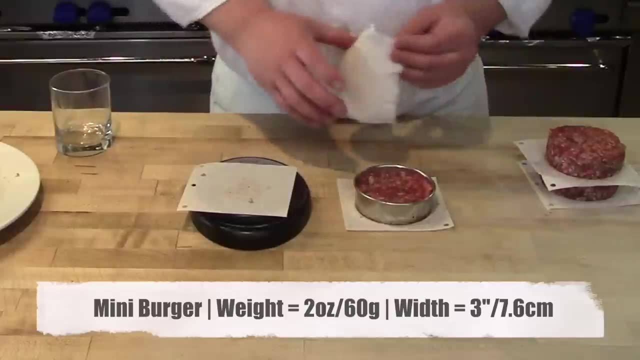 paper. Now, since this doesn't fill the mold to the top, we're going to use the bottom of a glass to smooth out the top of the burger And then we're going to press down using parchment paper. Now notice, as I am forming and handling these burger patties, I'm being as gentle as possible. 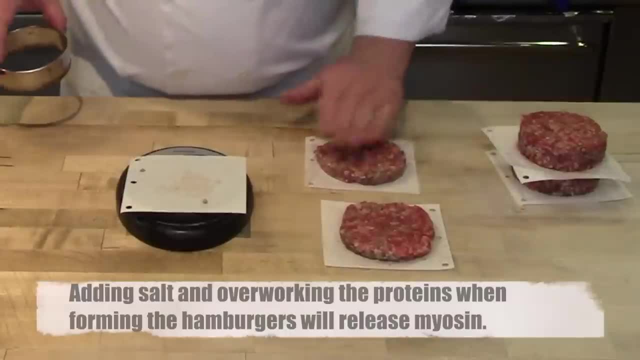 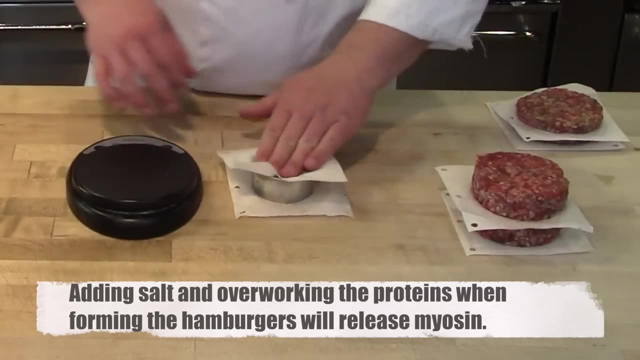 I'm not overworking them And I haven't added salt during this entire process. That's because overworking the proteins and adding salt is going to release myosin. The myosin will make the hamburger meat gluey and force it to stick together, giving you more of a sausage patty. 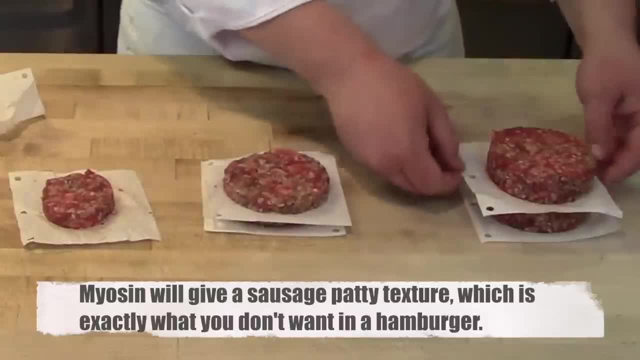 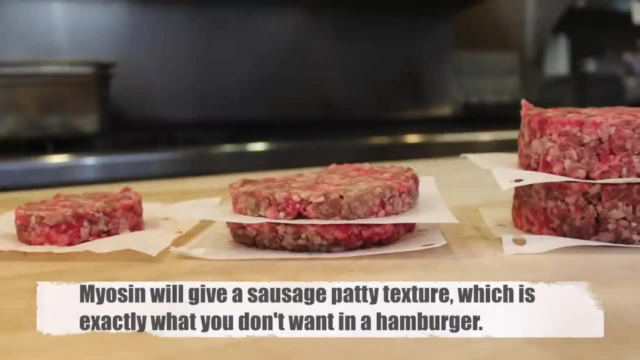 like texture, which you do not want in your hamburgers. So no salt ever. Use a gentle touch and just press your patty down Now, as I'm forming and handling these burger patties gently to form them, And you're going to have the best hamburger patties ever. 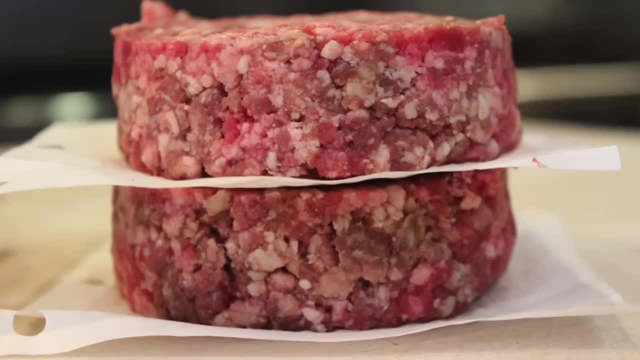 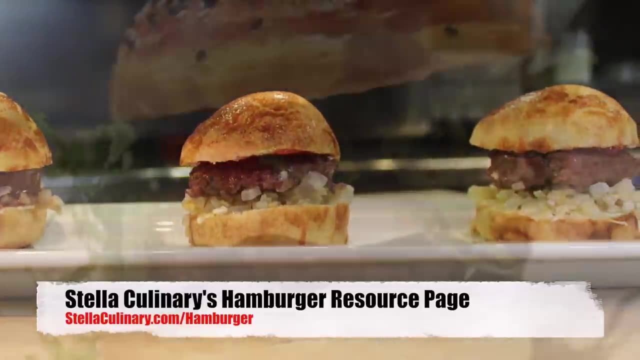 Now, of course, forming the perfect hamburger patty is just the first step in creating a great hamburger, And if you go to our new resource page, StellaCulinarycom slash hamburger, we're going to show you how to make sliders, how to make our large reversed seared eight ounce patty. 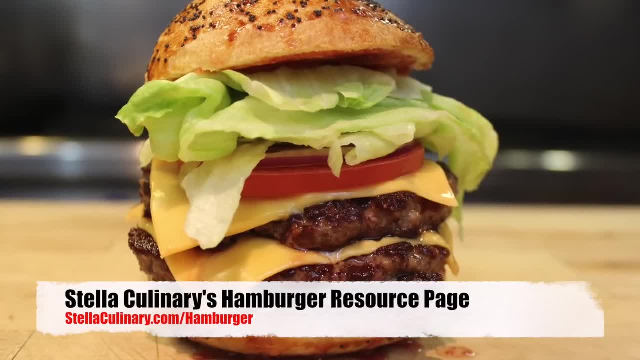 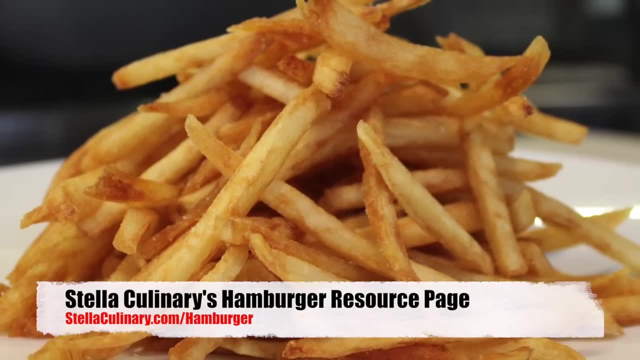 steakhouse burger, the double double, which is a classic. And of course, we have our recipe for our amazing hamburger brioche bun and even a couple of different French fries, including the classics, the seasoned and the best. So let's get started. 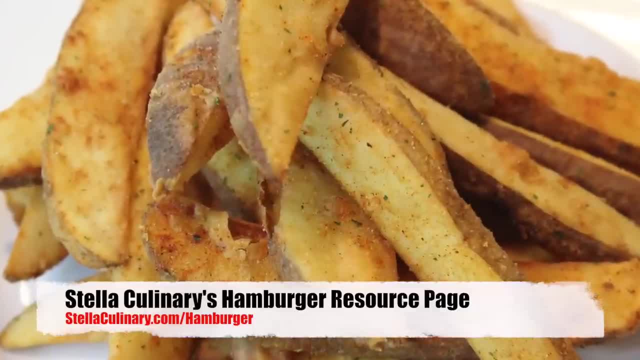 And the batter fried. So if you want to take your hamburger game to that next level, head on over to StellaCulinarycom: slash hamburger.